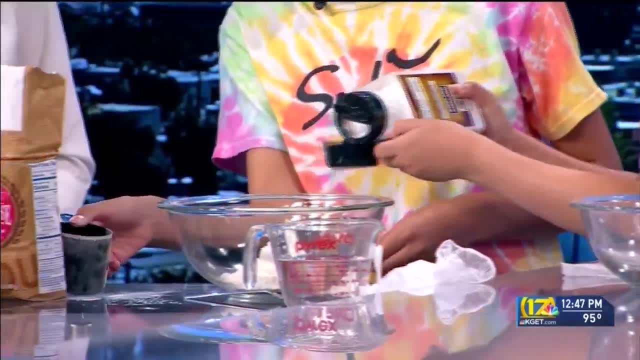 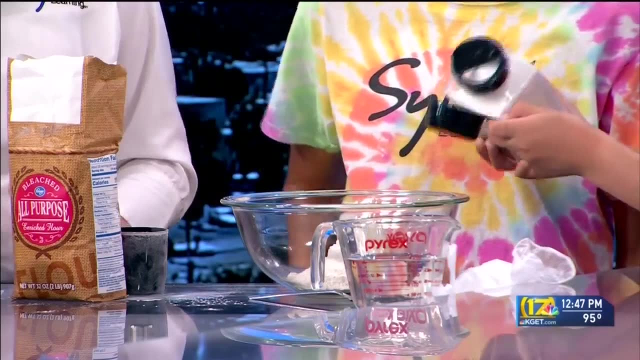 So we're going to put about a cup of flour And also a fourth of the salt. Now, this is sea salt, but it doesn't matter. if it's table salt, Okay. And when we have these two together, fill it up all the way. They don't create a chemical. 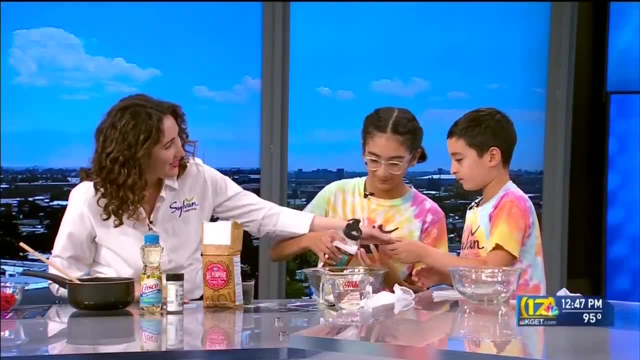 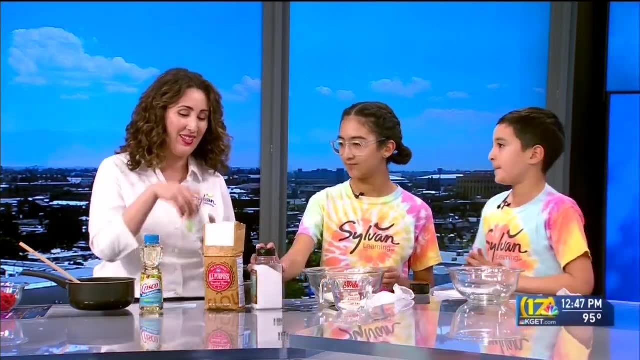 reaction. So this is what What is this called, Do you know? A mixture. A mixture, yes, because there's no chemical reaction in them. Really important also is to add in some cream of tartar. Oh, okay, Now this is found in the baking or the spices area of your local grocery store. You're 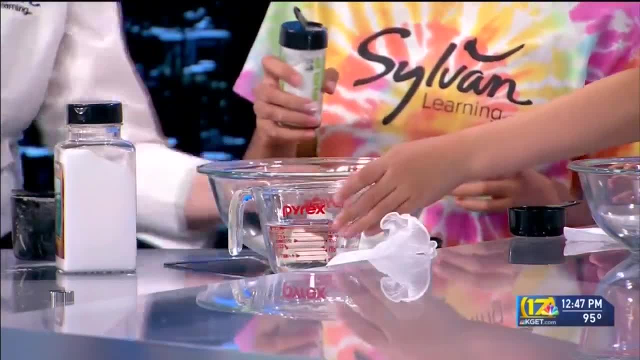 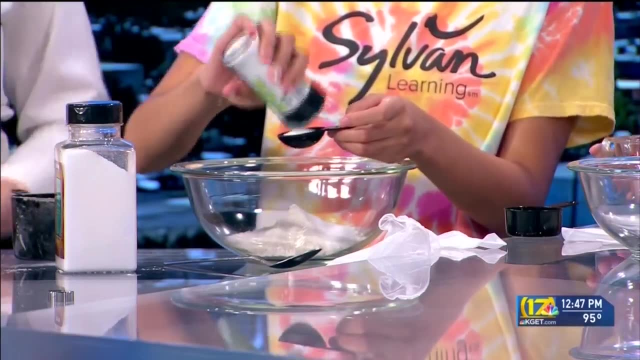 going to put Two tablespoons of that in. It's right in here, Meanwhile on another cup. What do you think that cream of tartar, by the way, does? It makes it really soft. It makes it soft, It keeps it very soft. So we're going to put two in there In another bowl. 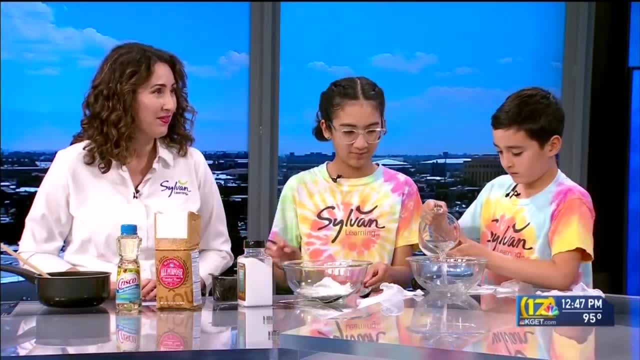 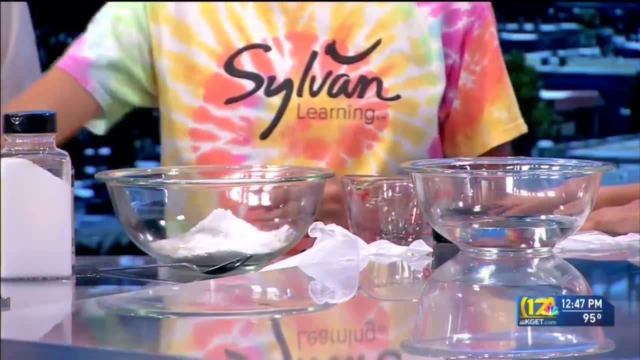 you're going to go ahead and put a cup of water. Warm or cold, does it matter? Yeah, I'd encourage warm, but if you want to speed up the process, at the end we might actually put it on the stove top, So it won't necessarily matter too much. We're going to put a tablespoon. 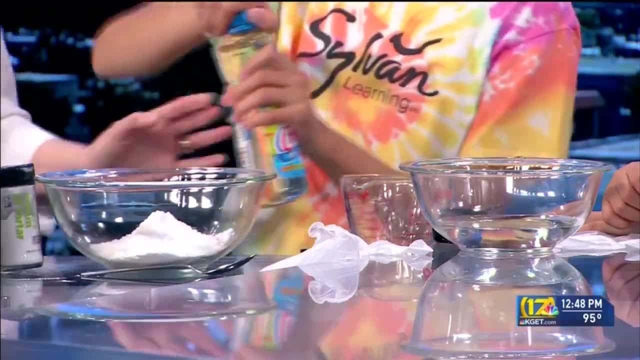 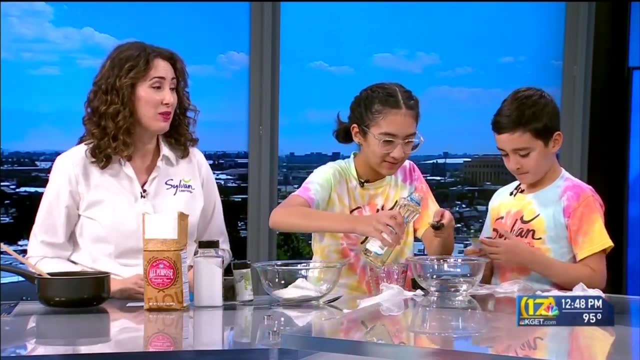 of oil, vegetable oil- A little tricky there Got it, No. And then, finally, we're going to add either some food coloring or, in this case, we're going to actually use a package of Kool-Aid. Oh fun, Just the powdered Kool-Aid, Powdered Kool-Aid. So, as you see, with the ingredients, 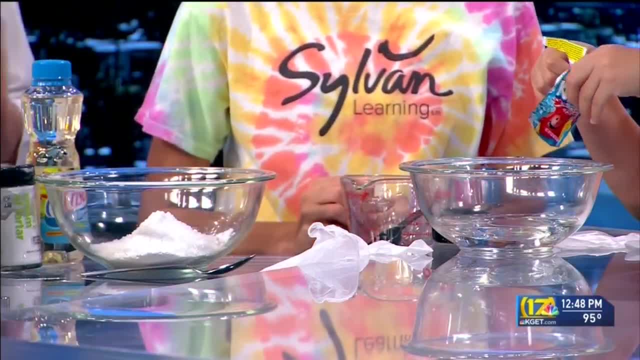 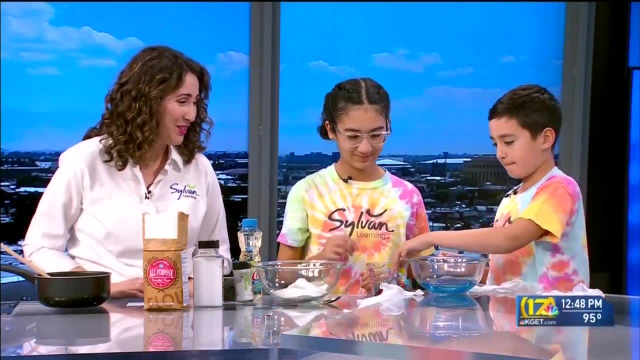 it's really non-toxic, It's edible, but I don't encourage it. Right, you don't want to fill a toddler belly with that, but toddlers tend to put everything in their mouth. It'll be very salty if you do so. definitely don't encourage that. 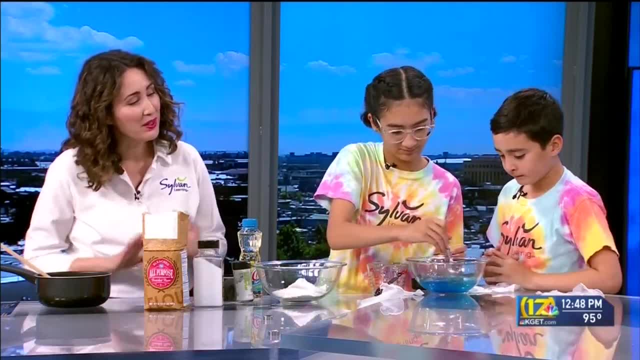 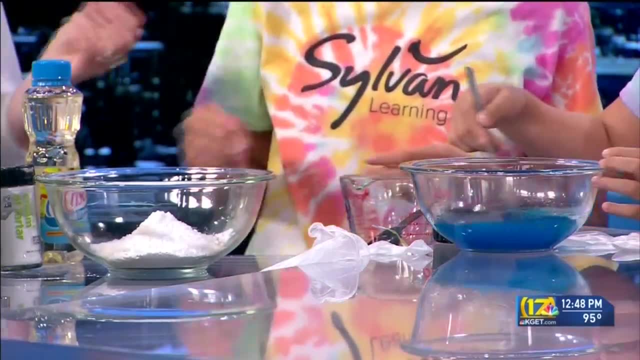 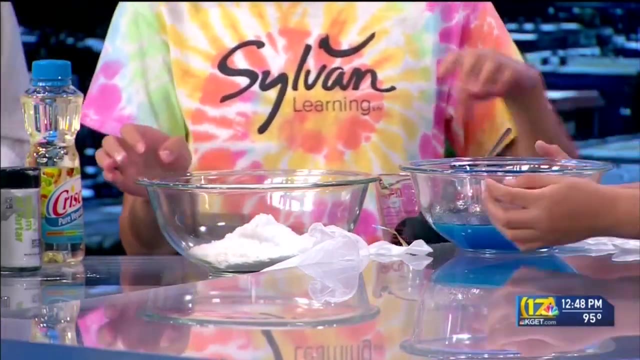 You'll mix those two together. You'll notice the oil and the water separate due to the density of the two. but what we're doing by mixing them once they become one, you're creating a solution, as opposed to the mixture. Okay, Now here's the messy part. We're going to place the two together. 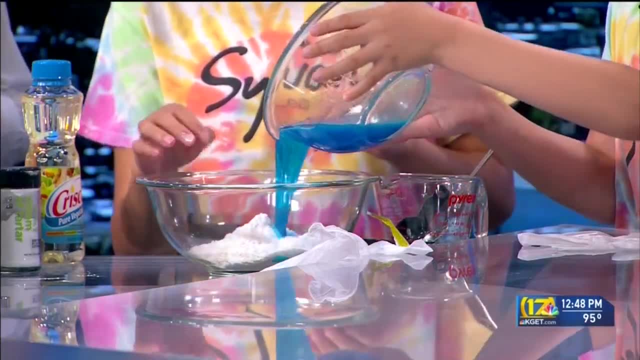 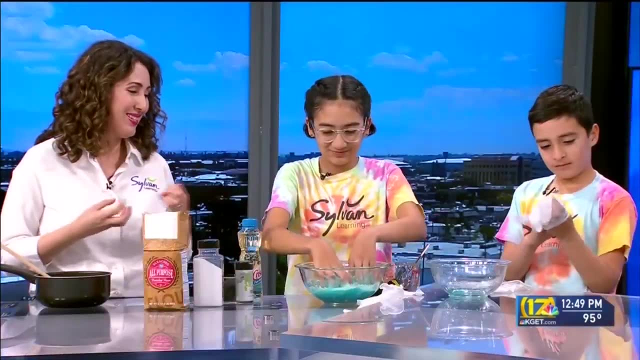 and you can either use your hands, go ahead to mix it up, or, if you want to get some gloves, you may do so. Okay, So that's where you begin to knead the mixture together so that you create a new substance.